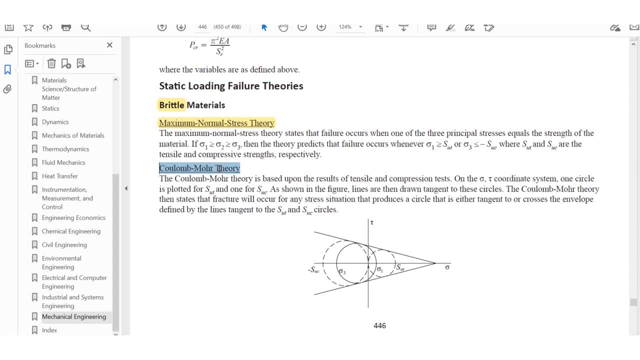 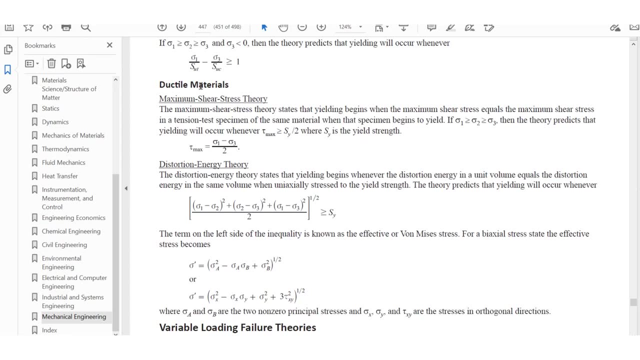 going to use the maximum normal stress theory or the Coulomb-Moore theory, which are both applicable for brittle failure. So once again, in the previous question we're focusing on ductile, Now we're looking at brittle and we're looking at static loading failure. 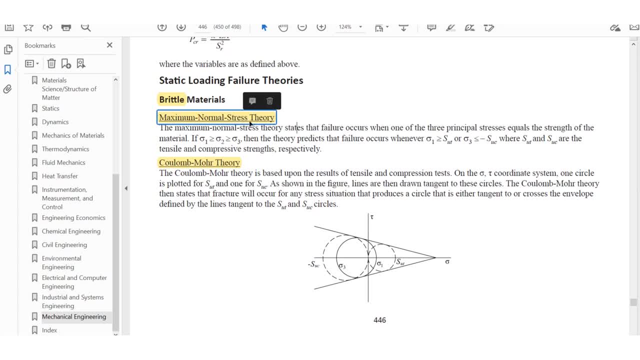 So we're going to focus on the maximum normal stress theory here, And we know that the maximum normal stress theory states that failure occurs when one of the three principal stresses equals to the strength of the material. So what we're doing here is we're taking a material, we're 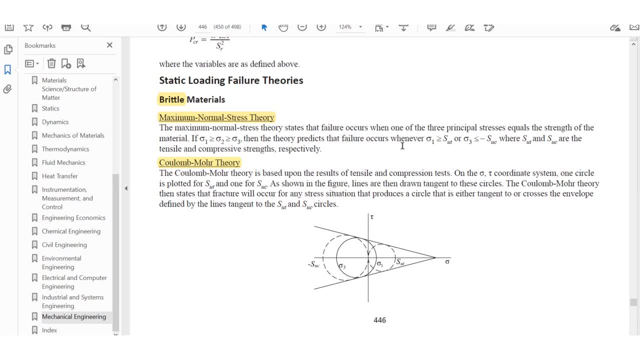 taking it in the lab. we're testing it for the ultimate strength, whether it may be intention or compression. Then, based on our three principal stresses that are applicable to the loading conditions we have, if one of these equals to the strength of the material, 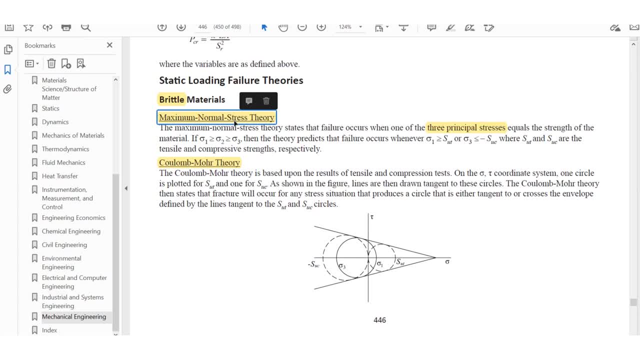 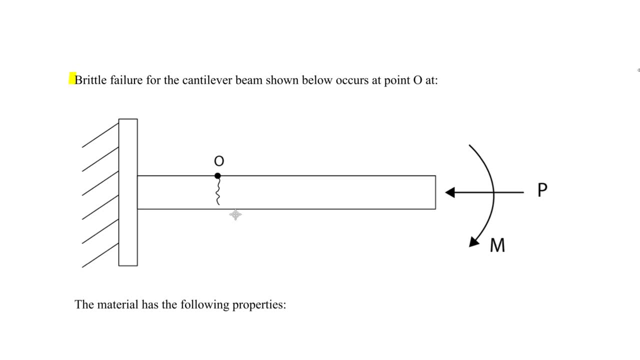 we know we have failure. That's all it says for the maximum normal stress theory. So if we go back to our question here, we're told that brittle failure. so brittle tells us we have to use those equations right, For the cantilever beam shown below occurs. 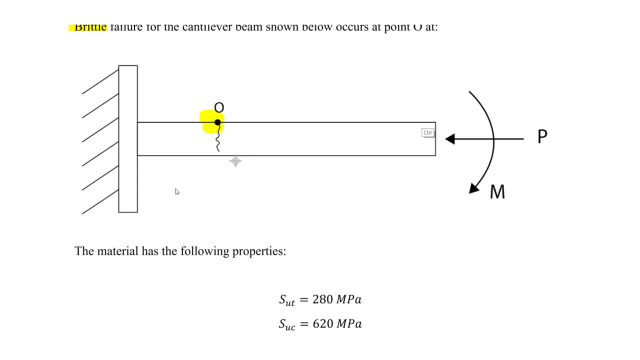 at point O. So we know we have point O, We have some crack in here, So we have. we're assuming it's brittle failure and it's strictly in the vertical direction. This is typical when you have a tension, brittle failure. So then we're told that the material 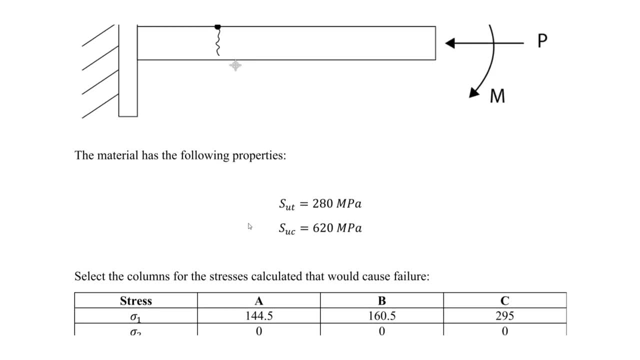 here has the following properties: So the ultimate, this SUT is going to be ultimate tensile strength. So ultimate tensile strength, And we know that the bottom is SUC, it's the ultimate compression strength. So that's all we have here And these are determined in the lab And what we want to. 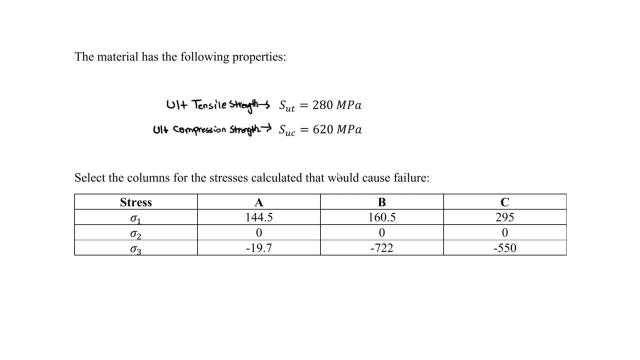 do here is select the columns for the stresses calculated that would cause failure. So we are trying to determine what would cause failure And we want to select the column- Is it this column, column A, or column B or column C, based on these principal stress conditions. 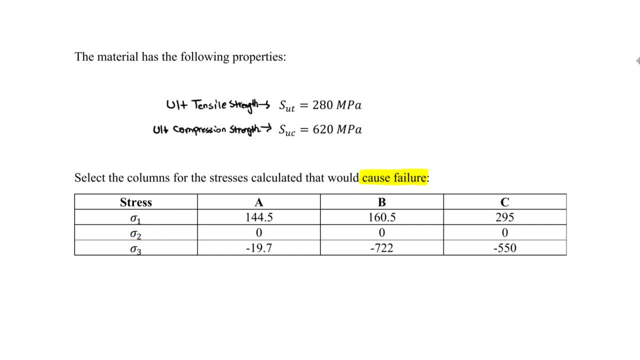 So these are the principal stresses we're given, And they're in order from greatest to the smallest. So sigma one is the biggest, We know sigma two is going to be zero. This does not change, but sigma three does change. So we have these and we want to select the. 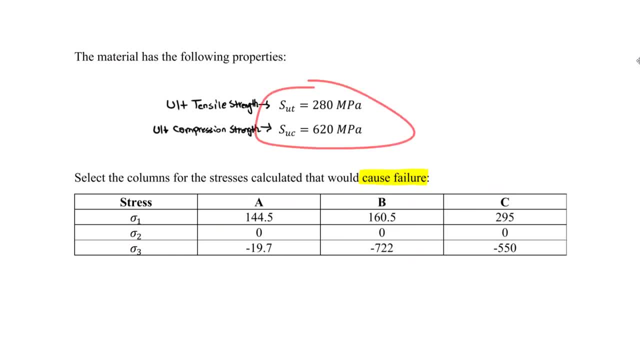 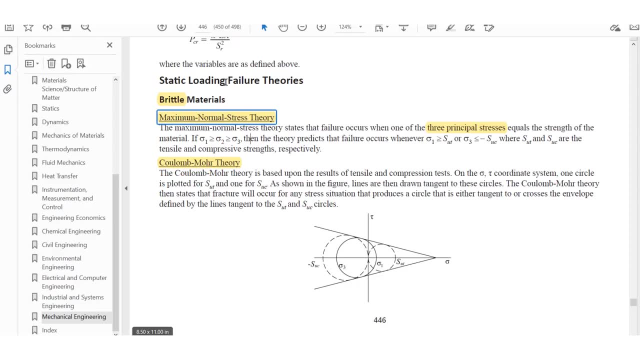 column. that would cause failure for the material, And we know we have a brittle material right. So what we can do here is apply that theory, the maximum normal stress theory. So let me quickly draw the Mohr circle here And what we have essentially is, let's say, on the x-axis, 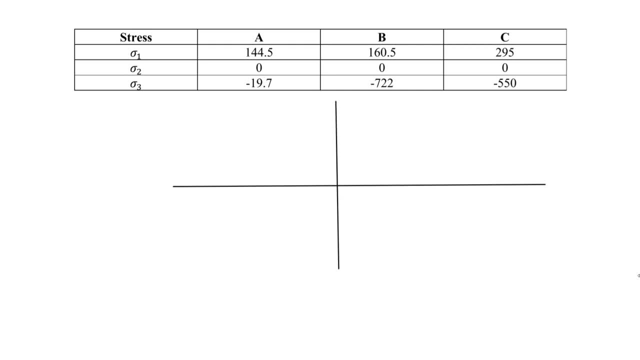 we have the stress On the y-axis, we have the shear, So tau on the x-axis is sigma. So we know we're at sigma one. Let's just look at A for the sake of visualizing this on the Mohr circle. Let's look at A. So 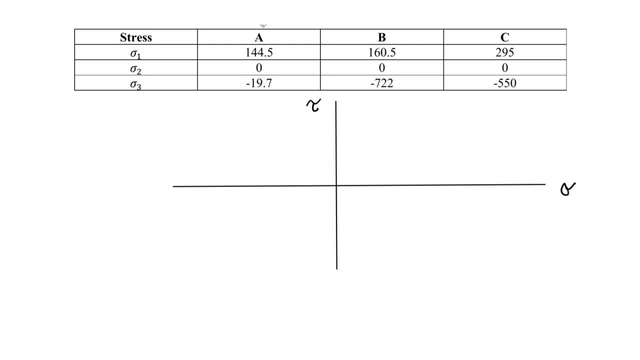 we know sigma one is around 144.. It's positive, So it's going to be somewhere here. This is our sigma one, And this equals to around 144.5 megapascals. And we know sigma three is going to be the negative 19.7.. So let's just say it's somewhere here, So it's sigma three. 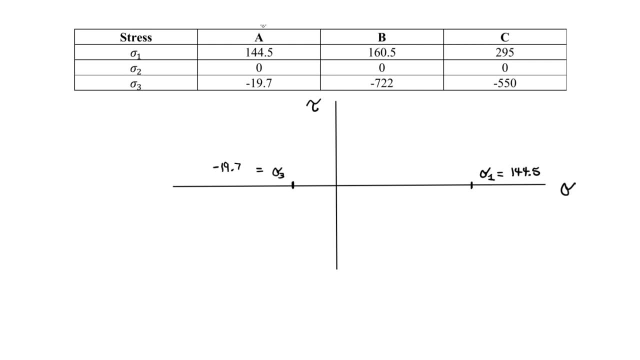 equals to negative 19.7.. And we know sigma two is zero. So it's just in the middle: Sigma two equals zero. So what we will have here is two circles. So we're going to have a circle. that's going to be- I'll use red. So we have one circle here and we know we're going to. 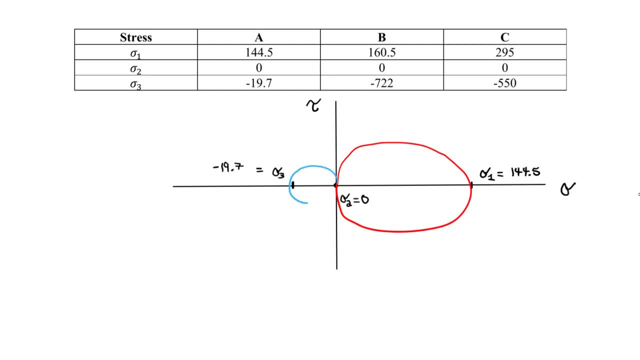 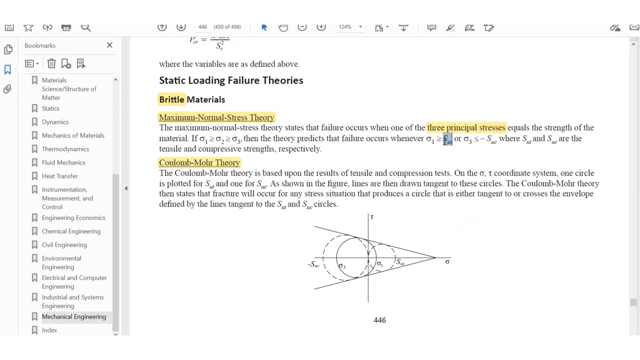 this other circle. we have two circles and we know we're gonna. these are going to be bounded by an envelope which we will talk about later and, based on these two circles, what we will do is essentially use the maximum normal stress theory and we want to test: is Sigma 1 greater than our ultimate tensile? 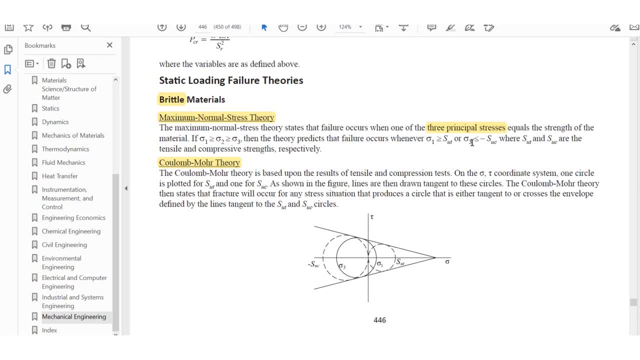 strength, or is Sigma 3 greater than it? essentially greater than this is still greater than our ultimate compression strength, or in other words, it's less than the ultimate compression strength, which is gonna be negative. we have to notice here that it's negative s ultimate compression, so it's gonna be. 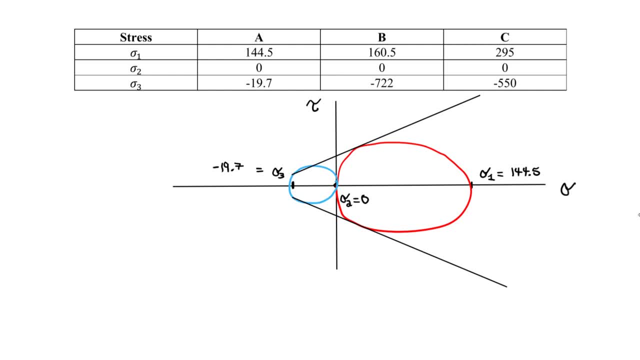 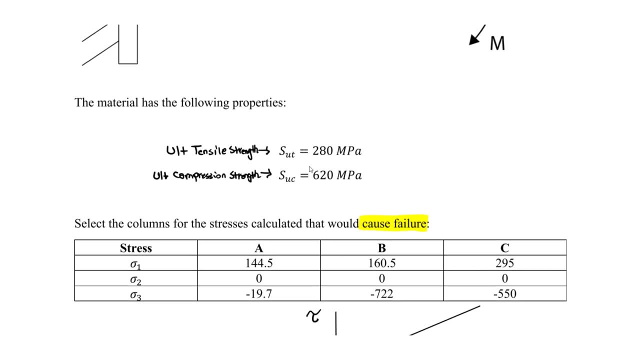 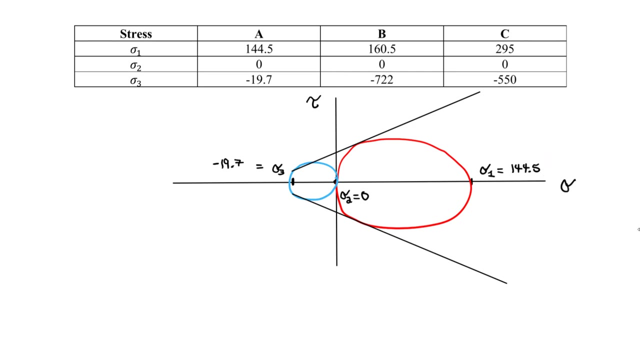 somewhere here. our ultimate compression, so let's plot that on the circle. so our ultimate tensile strength, saw strength based on these conditions, it's gonna be 280, so let's plot that here. 280 will be. I'll use this color. so this is 144, so 280. let's just say somewhere here this is s ultimate intention. 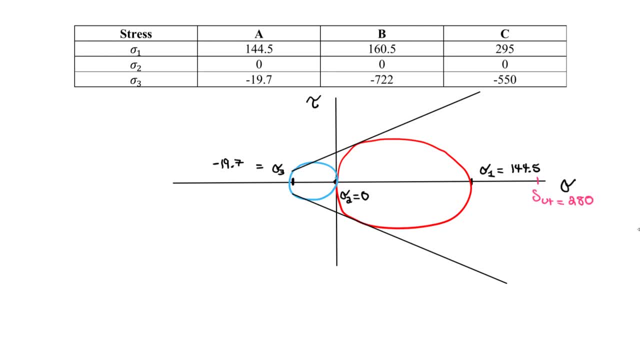 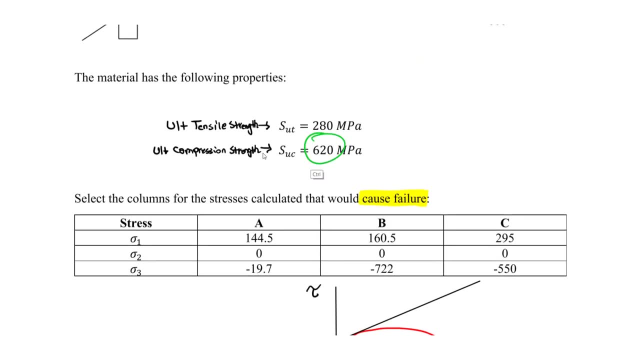 right, and this is 280. now let's look at the compression one. the compression one is gonna be the negative. right compression is negative 620. be careful here. they might not give you the negative on the FE. you just have to know the compression is always negative, just like what? 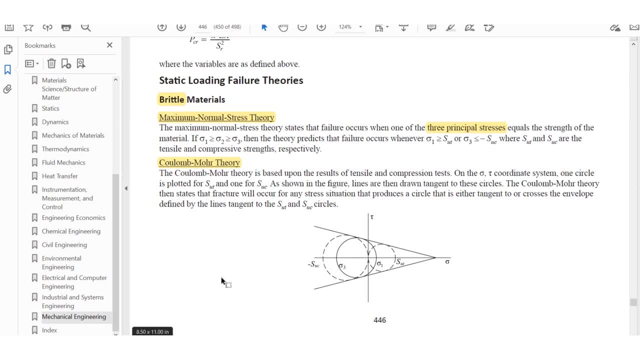 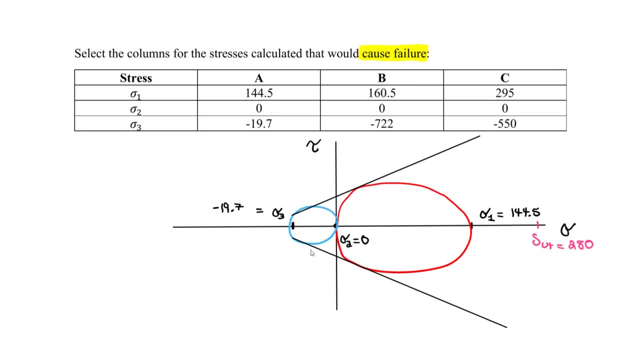 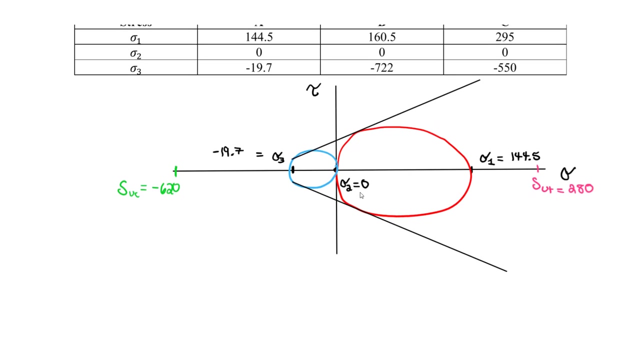 you're comparing here, they have this negative sign, so we have to plot it on the left side. so this is negative 620, so it's gonna be all the way here. so it's gonna be negative 620. and this is s. you see, ultimate compression strength. so what we do now is we know that if our Sigma 1 is somewhere, 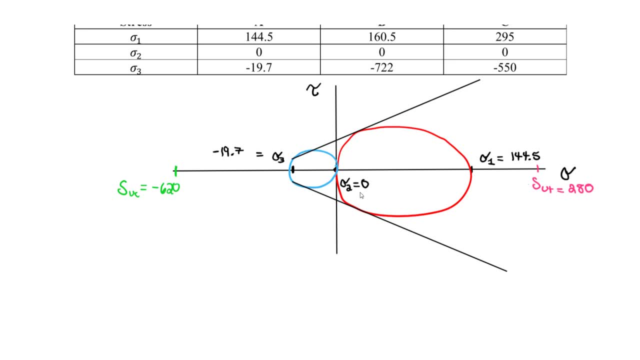 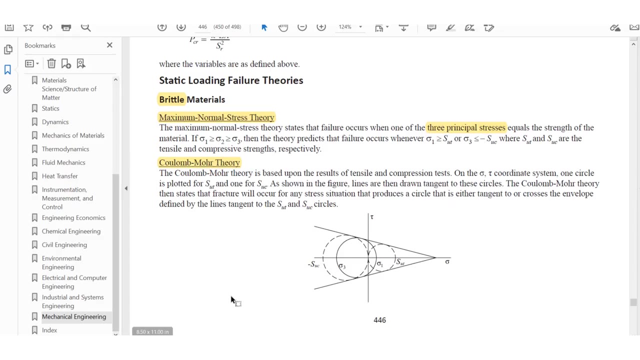 in this region and it crosses the ultimate, we know we have failure. and if Sigma 3 is somewhere behind here, we have failure. so let's look at column a and we're testing these conditions right. so Sigma 1 has to be greater than or equal to s ultimate. 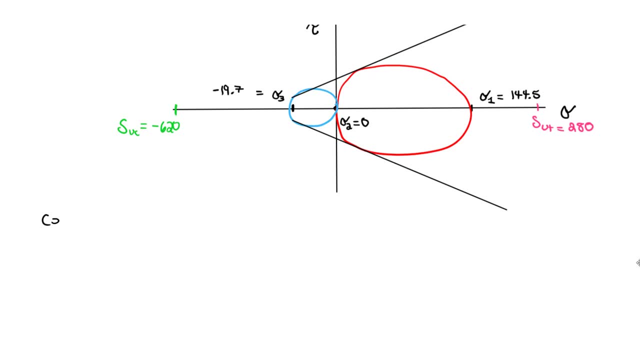 so we know that for column a, what we do is based on these. Sigma one has to be greater than or equal to, that s ultimate, and we know Sigma 1 is what it's going to be. we're looking at column a. it's gonna be enough. 144. 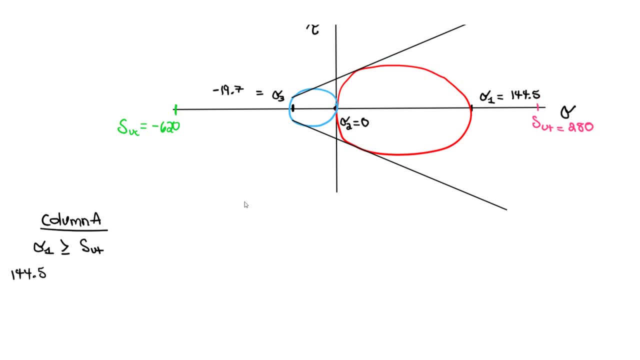 144.5. everything is in units megapascals, which is fine, and as you could be used to multiply it up a few times, we'll have to pick and choose to pick a few times and then it верa 144.5. everything is in units mega pascals, which is fine, and s you have to measure the force for the field. so it is 5.8 k's stopper, which is 4 whole. 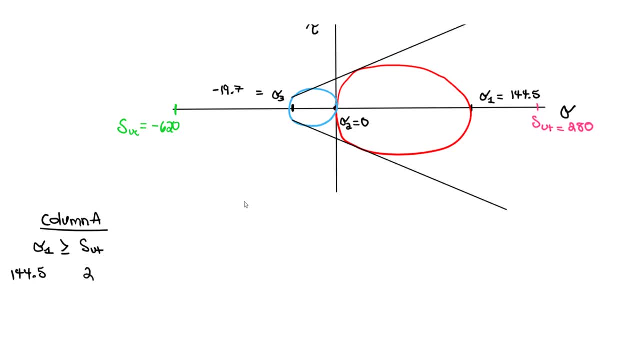 t is the ultimate. tensile strength is 280, right, and we know this is not the case, right? it's less than sigma 1 is less than 280. so we are okay, we do not have failure. we're okay, just like what we have in the figure here, since sigma 1 is less than s ultimate. we're looking specifically for this. 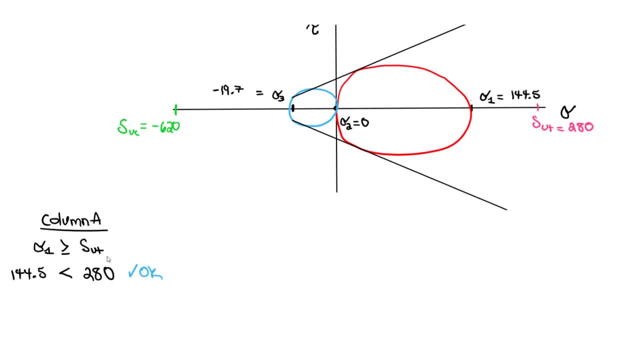 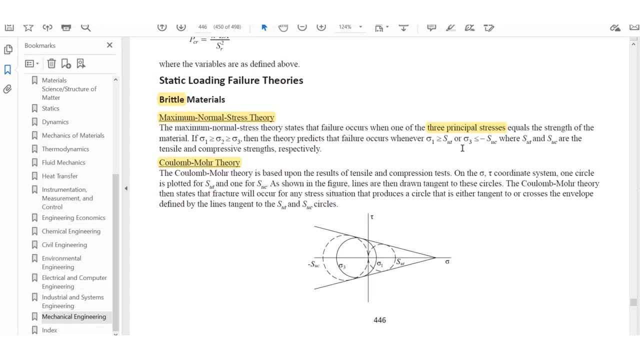 figure at column a right, and we know we're okay, we do not have failure. but we have to test the other condition and i believe that one is obvious if you look that sigma 3 has to be less than or equal to the negative s ultimate s, ultimate in compression, the ultimate compression strength. 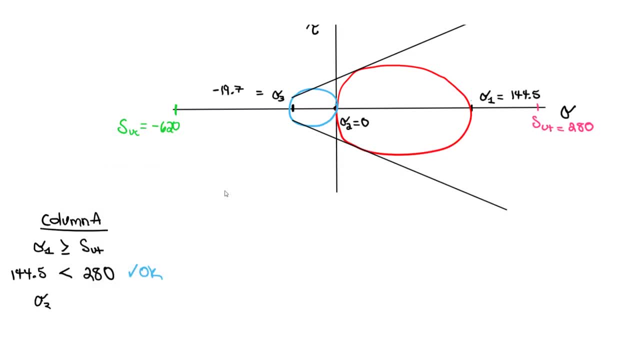 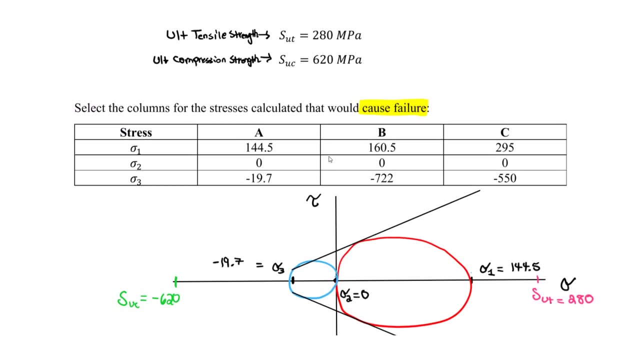 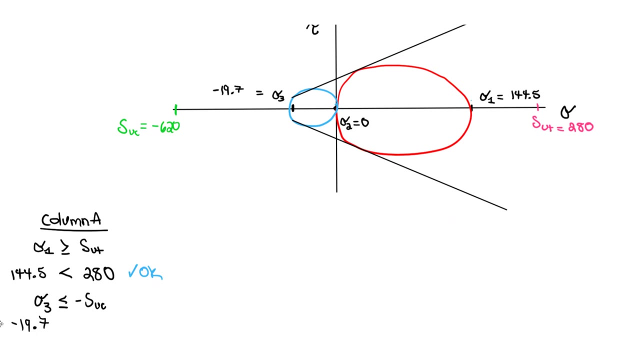 so let's test that. so sigma 3 has to be less than or equal to negative s uc. so we know sigma 3. i'm looking at this. it's going to be negative 19.7. so negative 19.7 and we know s uc. the ultimate compression strength is 620, so plug that on the right. 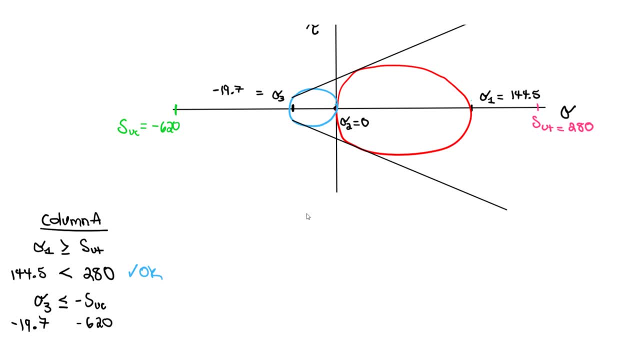 620 and negative 620. be careful there. so it's negative 620. so we know obviously this. the negative 19.7 is going to be greater than the negative 620. it's greater than right, it's not less than so it's somewhere here. we're not all the way out here. if we were here, we would 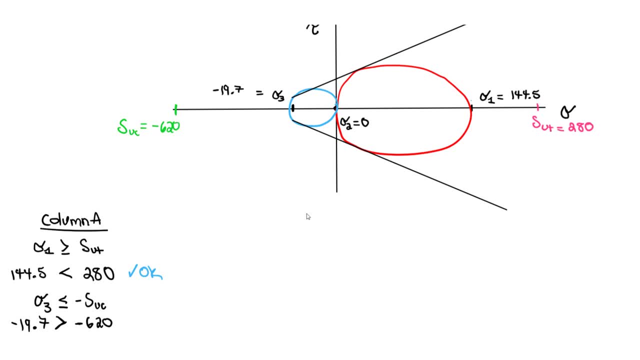 fail, right, so it's somewhere. it's greater than going to. the right is greater, right, so it's going to be greater than so we are okay. we do not have failure, so we're okay with that one. so that's all we have here. that's for column a. so we know column a. we're okay, so we do not have failure. 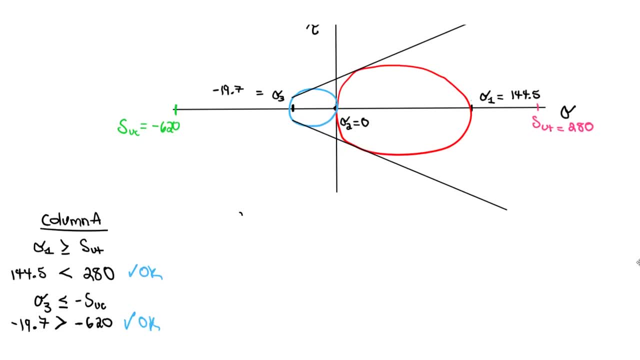 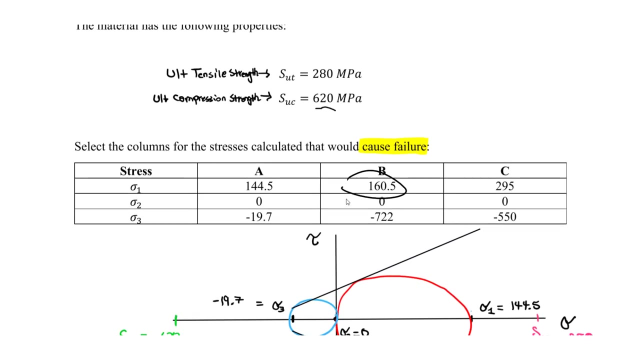 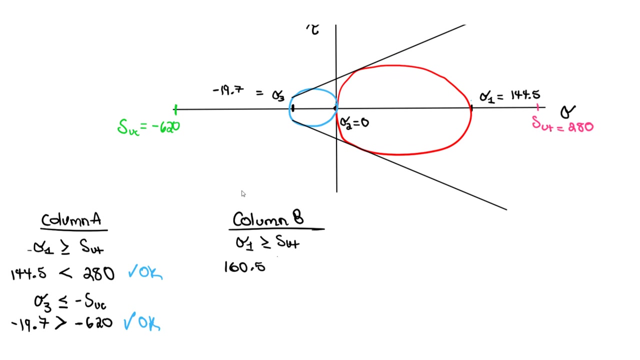 now let's look at column B. you do the same things, column B, and what we do is test this. so sigma 1 has to be greater than or equal to s? ut. what sigma 1 we're looking at? column B, it's going to be the 160, 160.5, and we know the ultimate tensile strength. 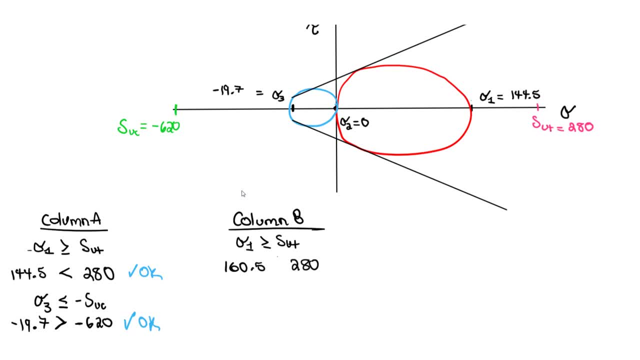 it does not change for the material. it's 280 given above. so we know that 280 is going to be bigger than that 160.5. so that's that. so we're okay for this one. so we're okay in tension, but we still have to test the compression. so the compression, sigma 3: 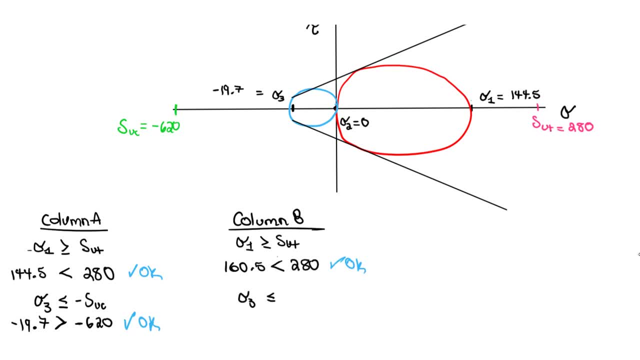 has to be less than or equal to the negative ultimate compression strength. what sigma 3 we're looking at, column B? column B is negative 7, negative 722, and we know that negative 620 does not change the ultimate compression strength for the material. but we know here, we realize that 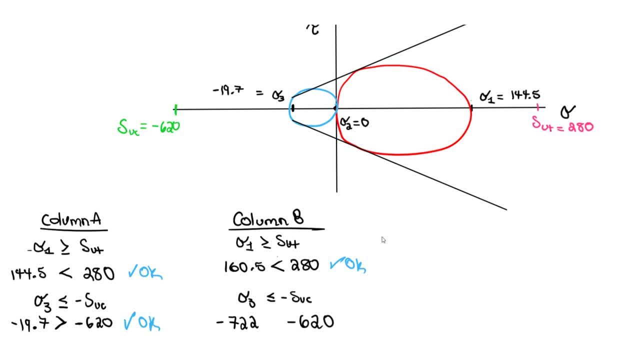 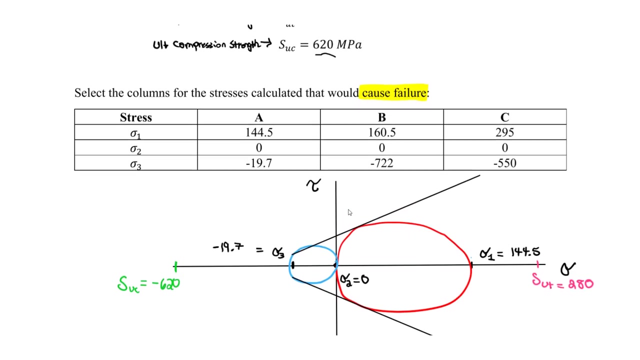 it is going to be that negative 620 is indeed greater than the negative 722, so it does meet this condition. so we do have failure. so we do have failure here. so we do fail- and this is specific- when we're looking at compression. so, column B, we do indeed fail, so let's choose that as an answer. 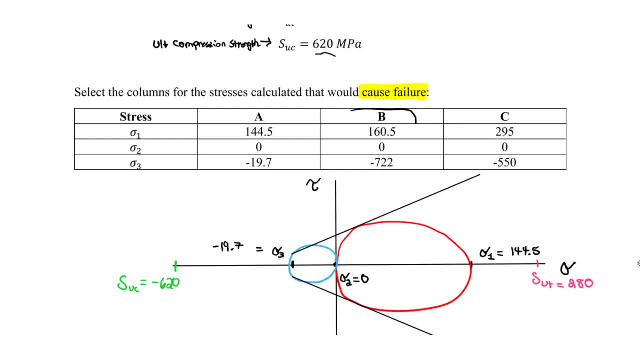 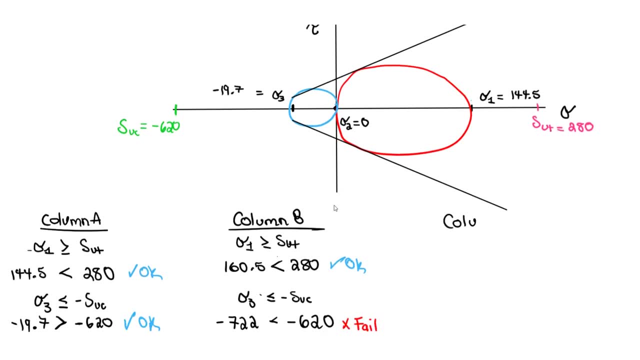 choice. so on the FE you would just select this column. so this is one answer that causes failure. and now let's look at column C. so you just apply the same principle, so you test the tension. first, the sigma 1 has to be greater than the ultimate tensile strength, and we know sigma 1 for column C is 295. plug in 295 on the left. the 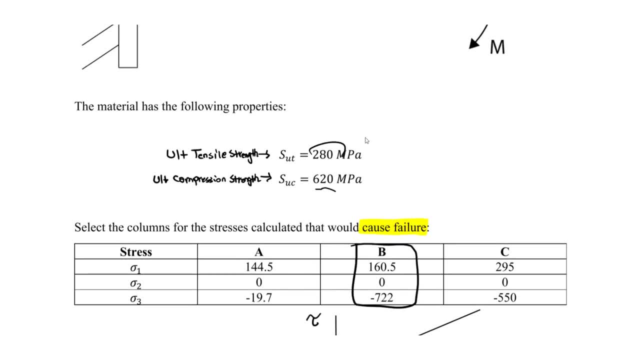 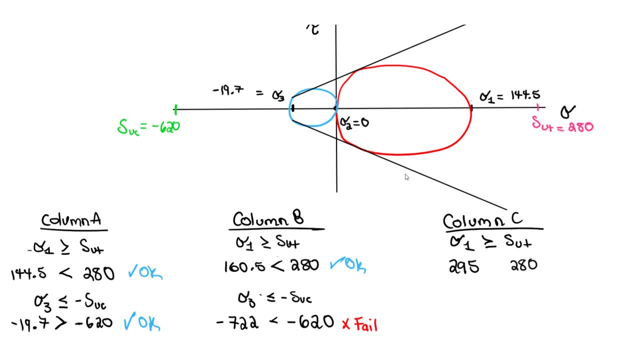 ultimate tensile strength does not change where. where do we get that? this should be given to you on that- for each 280 for the material. so we do have greater than the negative 620 and we know that is indeed greater than the 280. so it does meet the following criteria. so we do fail. so we do fail so. 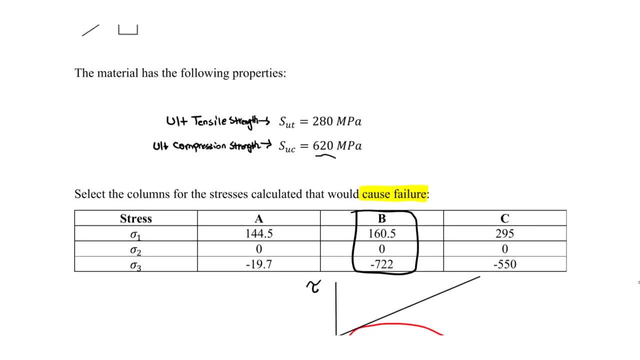 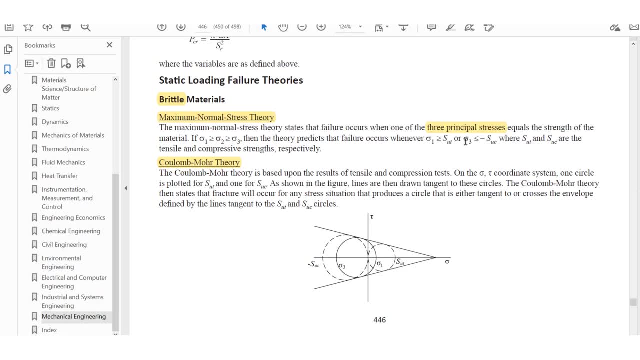 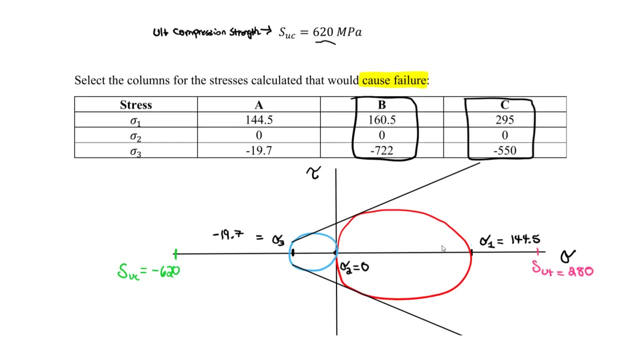 automatically. we know that column C does indeed fail, so you just have to have one of those conditions are criterion map in order to fill, because it says either we have this or this in order to have failure. so we know in this answer that we would select B. 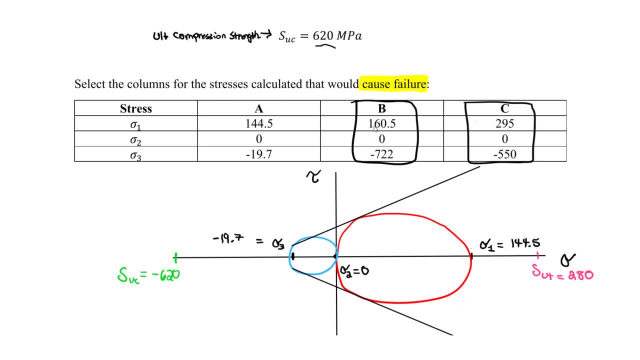 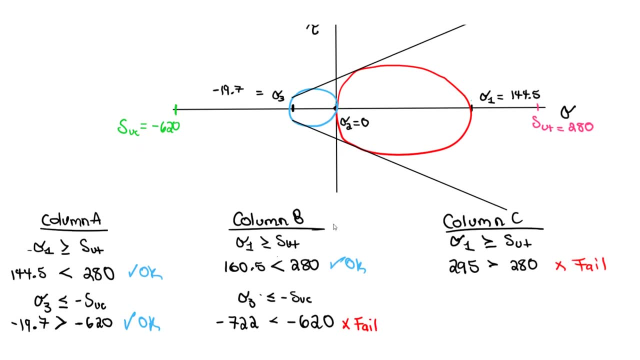 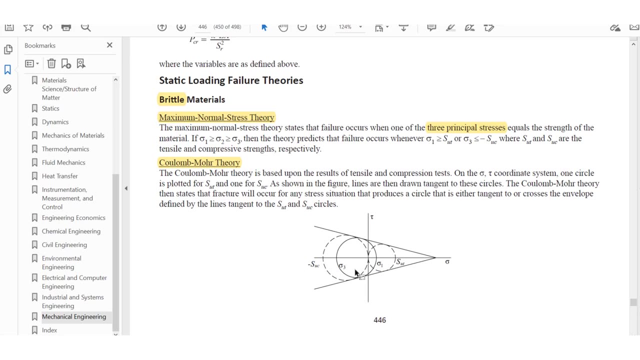 and C and that these are the principal stresses that would cause failure, and we're specifically looking at birth of failure using the maximum normal stress theory. so if we wanted to use the other theory, the cool on more theory, you- we would get the same answers. so we know we have an envelope here and we know that. 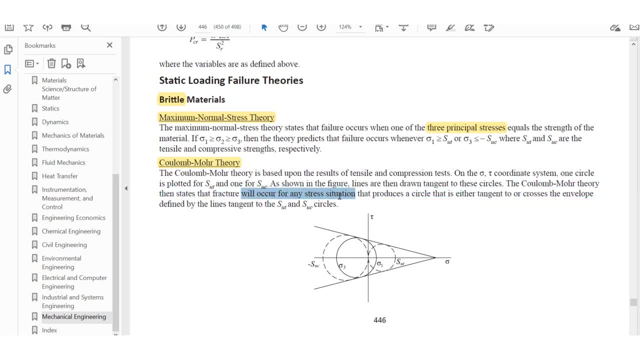 the cool on more. theory states that fracture will occur for any stress situation that produces a circle that is either tangent to or crosses the envelope defined by the lines tangent to the ultimate, the ultimate tensile strengths and the ultimate compression strength circle. so that's what that says. 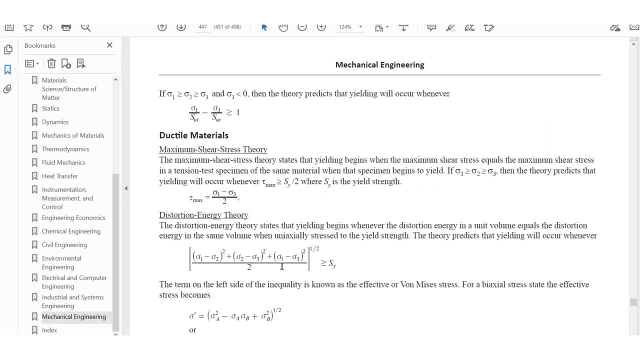 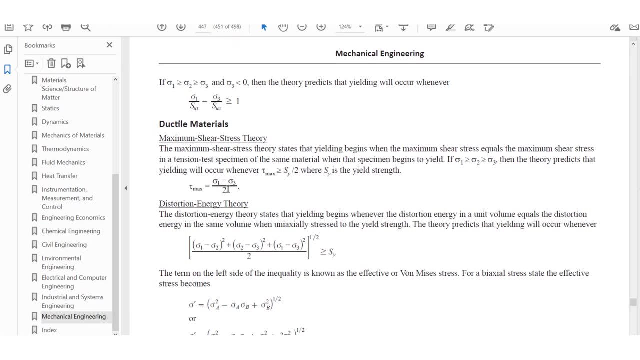 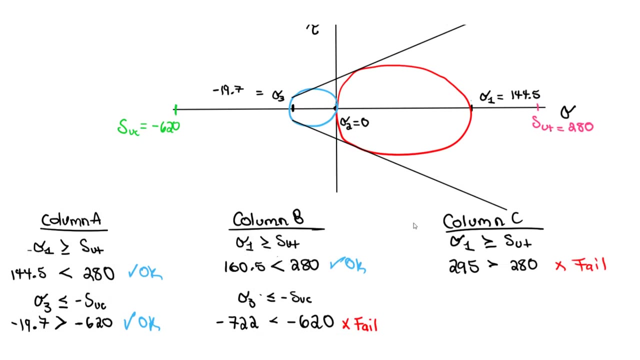 and we can test that using this envelope and which we did draw approximately here, the envelope, and what all you have to do for the cool on more theory is use these equations. so let's use that equation real quick for the sake of finishing this question. so let's do for column C specifically, I want to see: does it indeed fail, and does 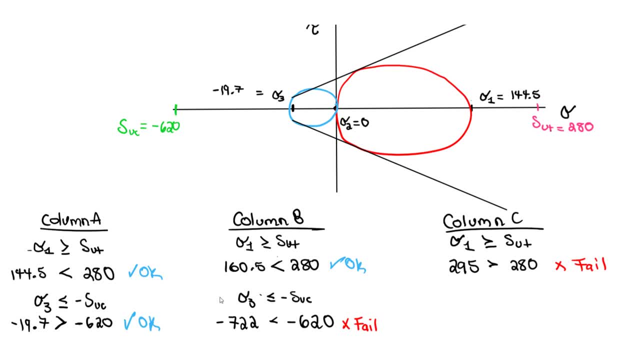 it confirm what we got from the other theory, the maximum normal stress theory. so all we have to do is use that equation. so we take Sigma 1 over Sigma ultimate. so let me write that: Sigma 1 over S ultimate, sorry intention, minus our Sigma 3 divided by our s ultimate and 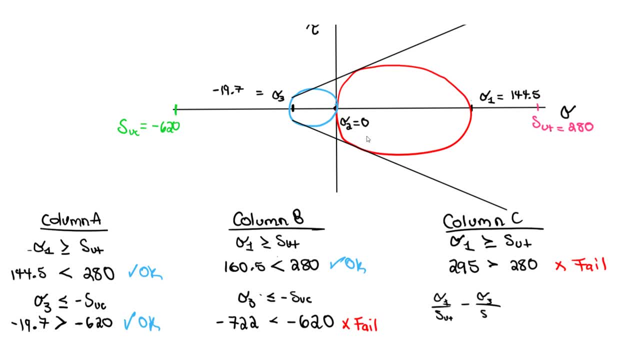 compression right, Sigma 3, divided by rs ultimate and compression, and we know this has to be greater than or equal to 1 for yielding or failure to occur. so if we plug, plug in what we have, Sigma 1 is can be 295. I'm looking at Colum C and we 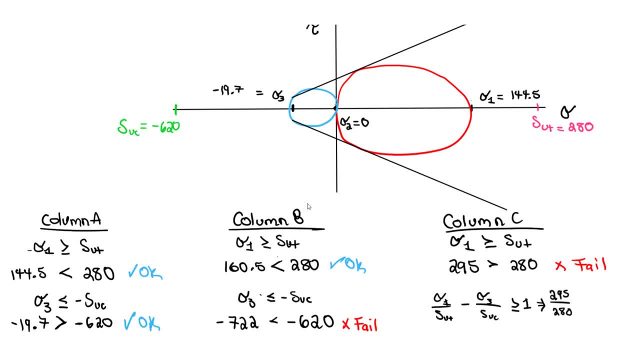 have Osseous, ultimate is going to be 280. here we have the kernel one, followed by Yeov died 1 S ontem, 280. then we do minus our sigma 3, is what sigma 3, we know, is going to be this negative 550. 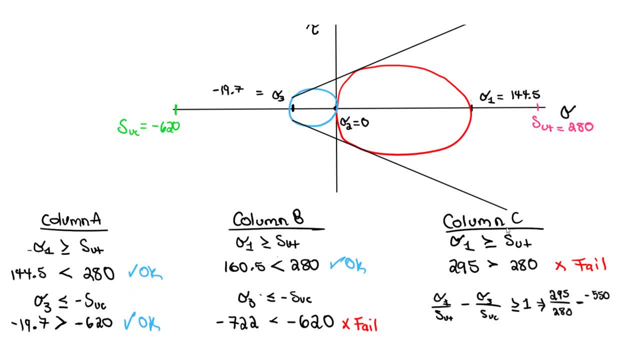 so keep that negative negative 550 divided by our s ultimate in compression. our ultimate compression strength is 620. so you can do the math for this and let me do it real quick. on my calculator you do 295 divided by 280, minus negative 550. be careful there. the s ultimate